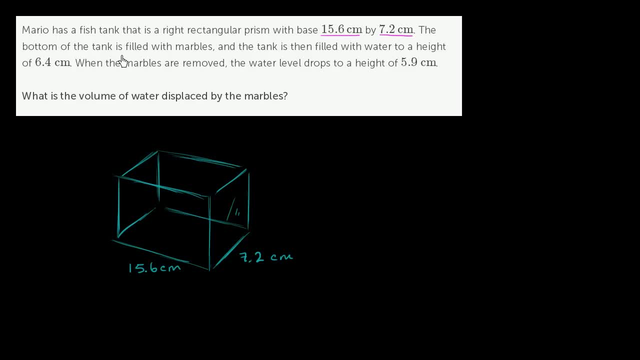 There you go. That looks nice, All right. the bottom of the tank is filled with marbles, And the tank is then filled with water to a height of 6.4 centimeters. So the water is filled to a height of 6.4 centimeters. 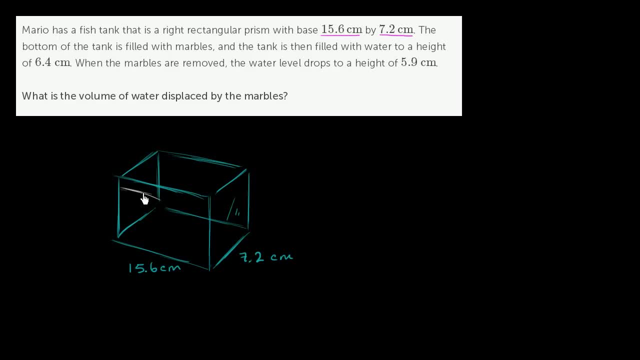 So this is the water when it's all filled up: 6.4 centimeters. So let's draw that And I'll make the water. well, maybe I should have made it a little more blue than this, But this gives you the picture. 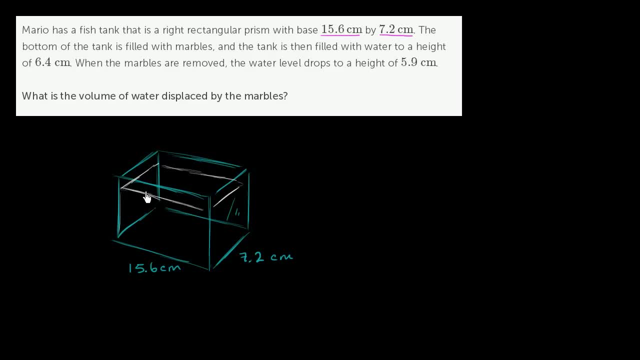 So the height of the water right over here- actually- let me do that in a blue color- The height of the water right over here is 6.4 centimeters. So that means that the distance from the bottom of the tank to the top of not the tank but to the top of the water- 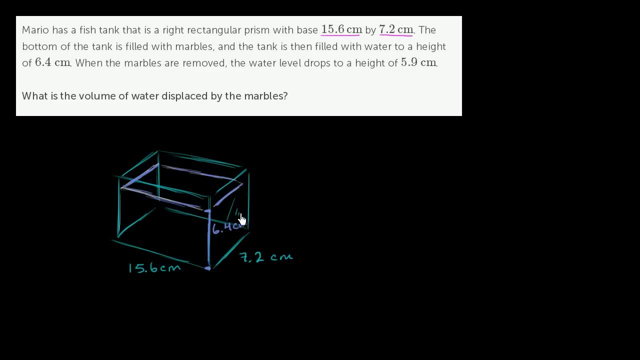 is 6.4 centimeters. 6.4 centimeters, Fair enough. So that's the top of the water. When the marbles are removed- and it started off with some marbles on the bottom- They don't tell us how many marbles. 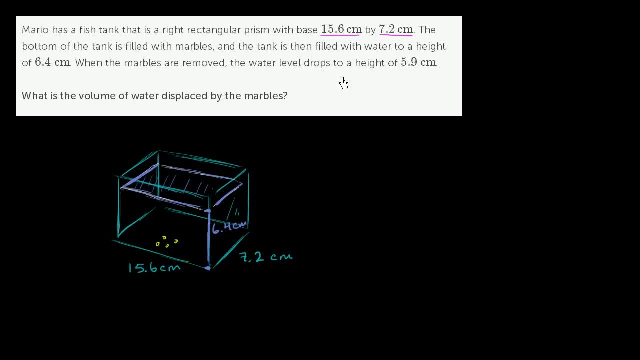 When the marbles are removed, the water level drops to a height of 5.9 centimeters. So when they're removed, the water level drops by a little bit to 5.9 centimeters. So it drops to 5.9, from 6.4 to 5.9 centimeters. 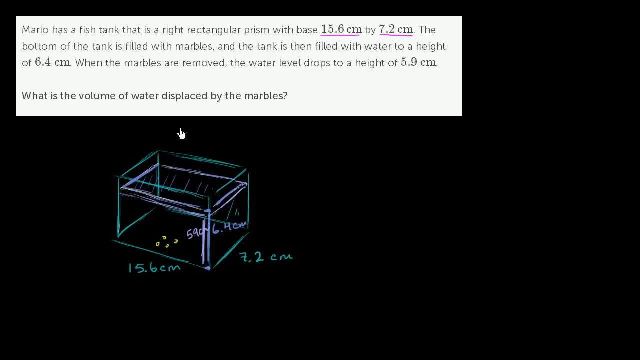 What is the volume of the water displaced by the marbles? So when you took the marbles out, the water dropped from 6.4.. So it dropped from 6.4 centimeters Down to 5.9 centimeters. 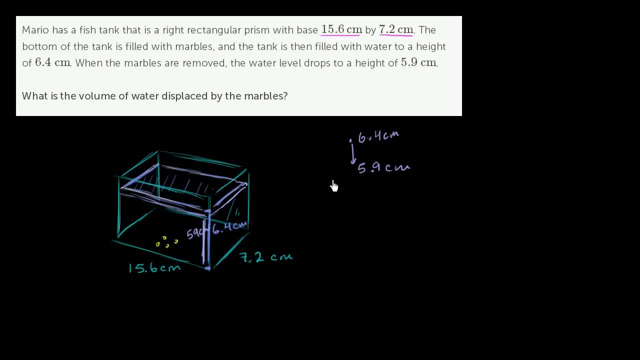 So how much did it drop? Well, it dropped 0.5 centimeters. So it dropped 0.5 centimeters. So what does that tell us about the volume of water displaced by the marbles? Well, the volume of water displaced by the marbles. 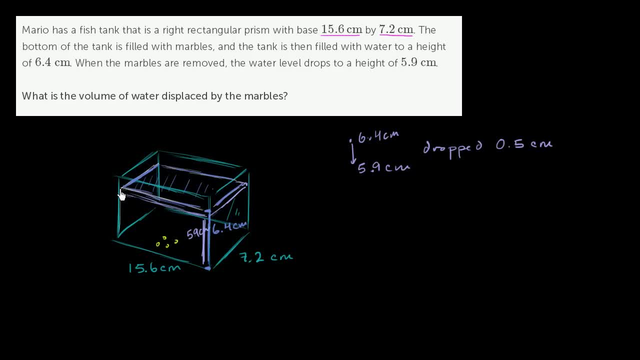 must be, the amount of must be equivalent to this volume, this volume of this- I guess this is another expression. OK, This is a rectangular prism. That is where the top area is the same as the base of this water tank, and then the height. 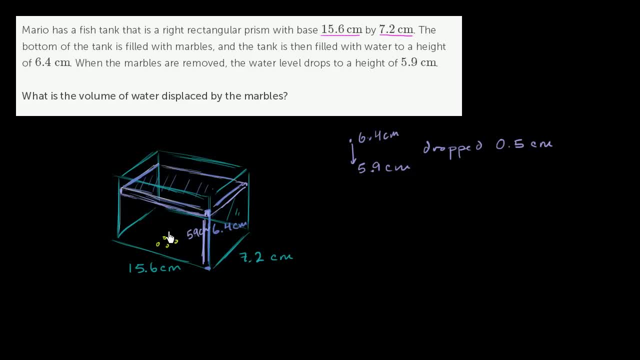 is the height of the water drop. When you put the marbles in, it takes up more volume. It pushes the water up by that amount, by that volume. When you take it out, then that volume gets replaced with the water down here. 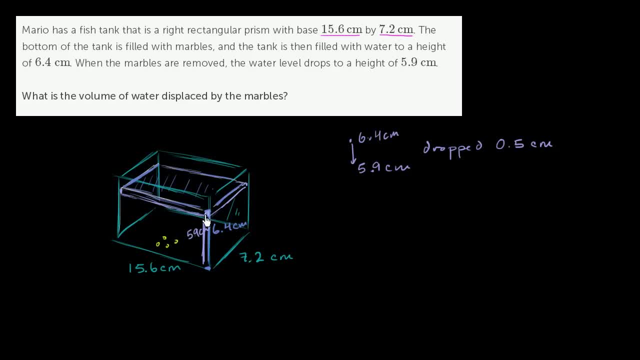 And then that volume goes back down. The water level goes down to 5.9 centimeters. So we're essentially trying to find the volume of of a rectangular prism, that is, that is equal to: so it's going to be 15.6 by 7.2 by 0.5.. 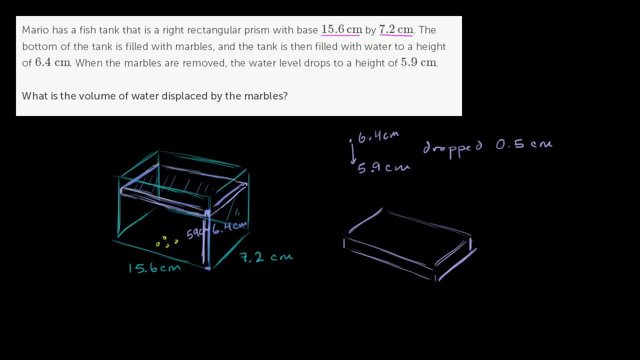 And I haven't drawn it to scale yet, but I want to see all of the measurements. So it's going to be 15.6 centimeters in this direction. It's going to be 7.2 centimeters in this direction. 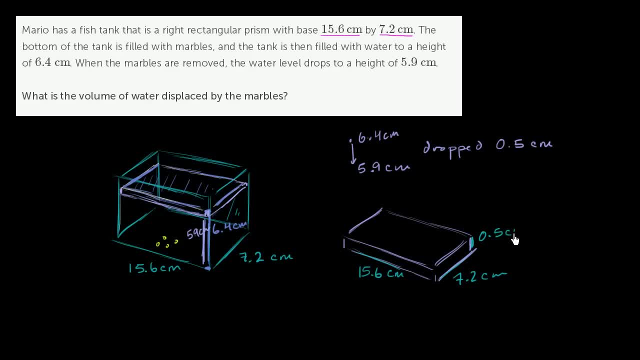 And it's going to be 0.5 centimeters high. 0.5 centimeters high. So we know how to find volume. We just multiply the length times the width times the height, So the volume in centimeter cubed. 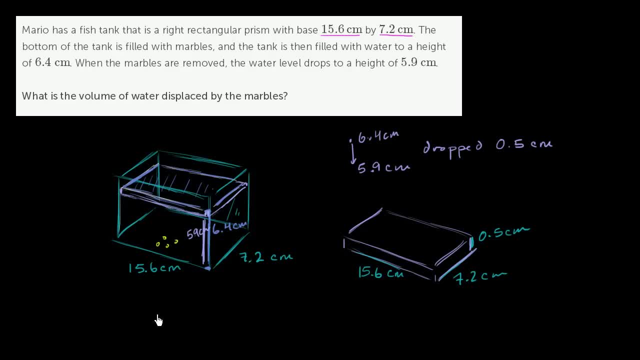 and we're multiplying centimeters times centimeters times centimeters. So it's going to be centimeters. cubed is going to be- let me write this down: the volume is going to be 15.6 times 7.2 times 0.5.. 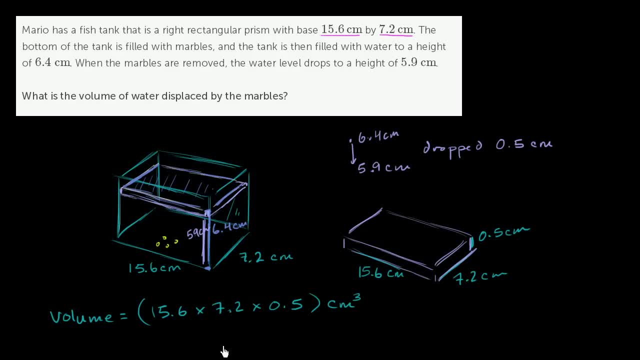 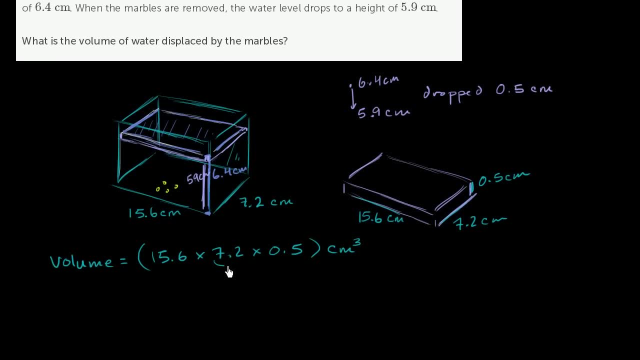 That's going to be in centimeters, cubed Cubic centimeters, I guess we could call them. Well, let's first multiply 7.2 times 0.5.. We can do that in our head. This part right over here is going to be 3.6, essentially. 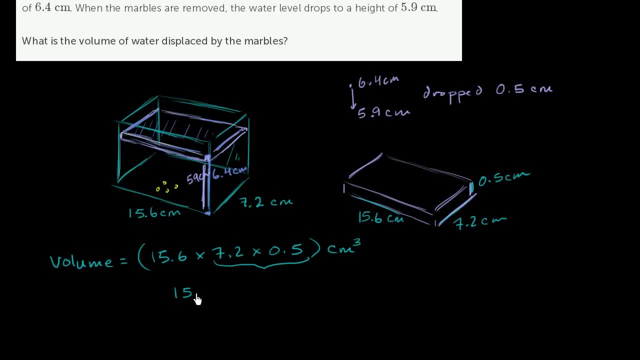 just half of 7.2. So then this becomes 15.6 times 3.6.. So let me just multiply that over here, So 15.6 times 3.6.. So I'll ignore the decimals for a second. 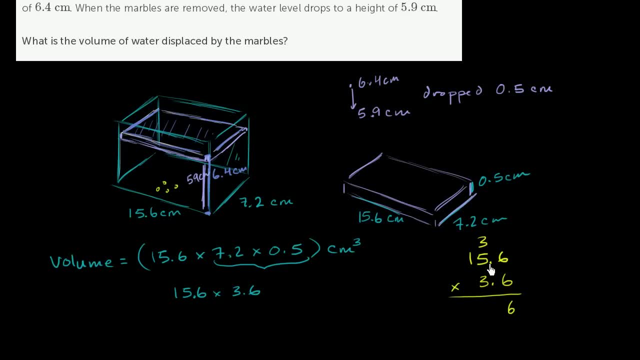 6 times 6 is 36.. 5 times 6 is 30. Plus 3. 3 is 33.. 1 times 6 is 6, plus 3 is 9.. And then let's place a 0 here. 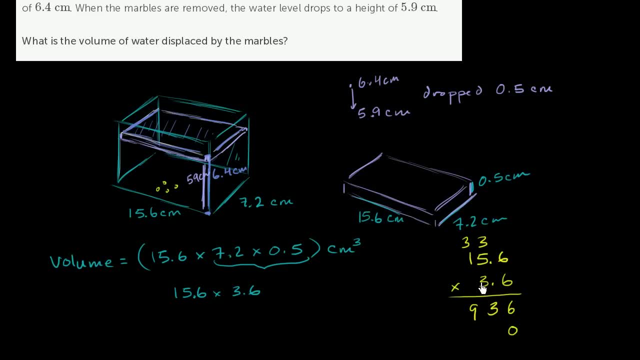 We're down in the ones place, but I'm ignoring the decimals for now. 3 times 6 is 18.. 3 times 5 is 15, plus 1 is 16.. 3 times 1 is 3, plus 1 is 4..